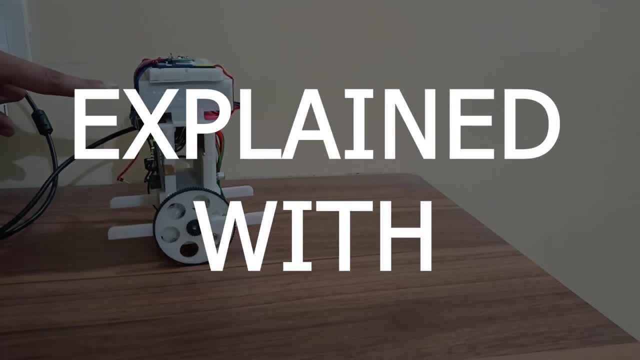 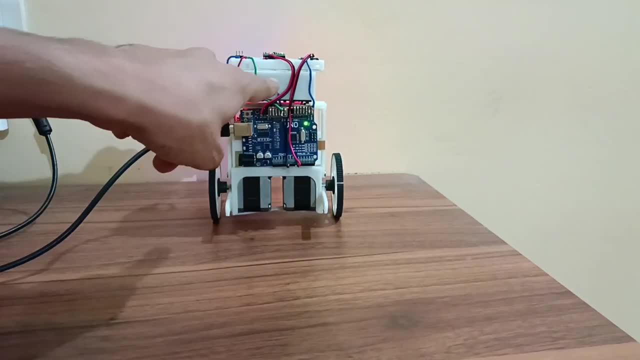 Let's talk about PID control. Chances are you've interacted with something that uses a form of this control law, even if you weren't aware of it, And so it's worth learning a bit more about what this control law is actually doing and how it helps us. We start with example of self-balancing robot. 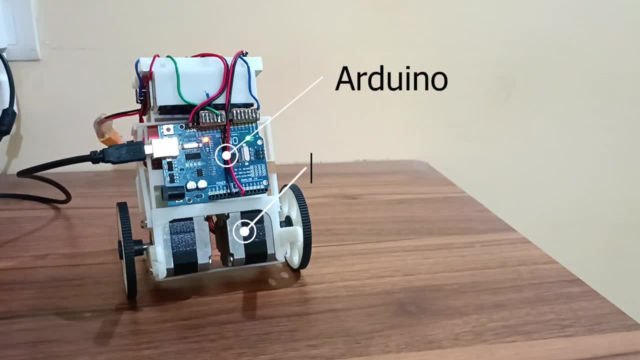 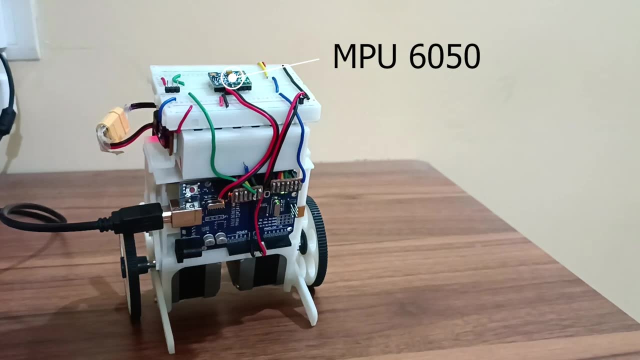 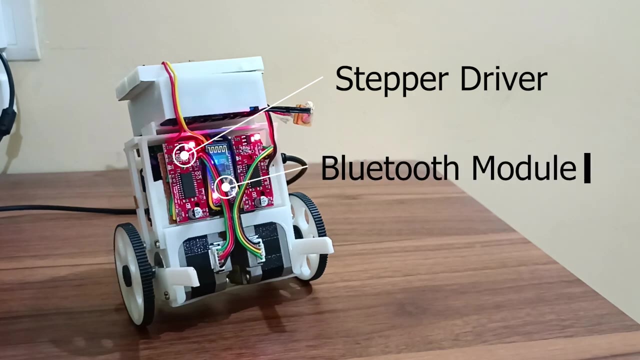 Here we have an Arduino Uno microcontroller, Stepper motors, MPU6050, 6-axis gyro plus accelerometer sensor for tilt detection, Stepper driver and HC05 Bluetooth module In self-balancing robot. we want the robot to stand on two wheels vertically. 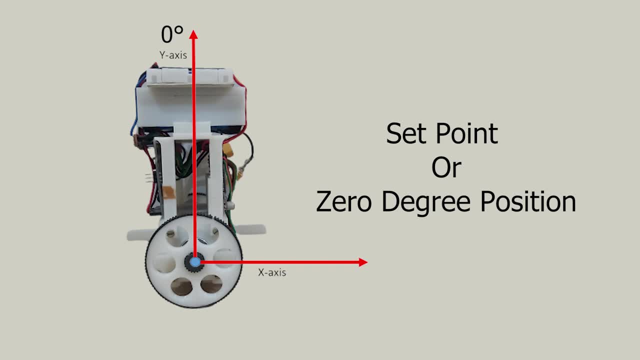 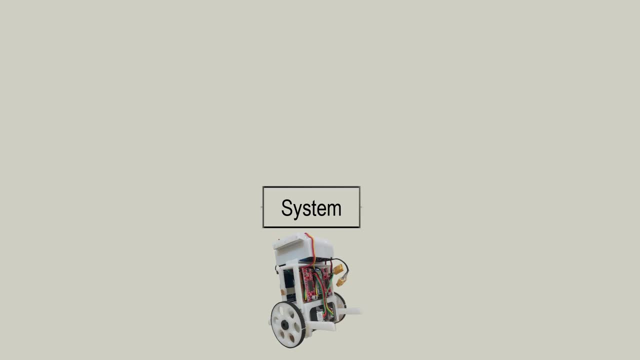 upright. Let's call this vertically upright position, the set point, or zero degree position. This is what we call the system that we want to control. The input into this system is the motor speed and direction, and the output variable is the robot's angle of tilt. The basic. 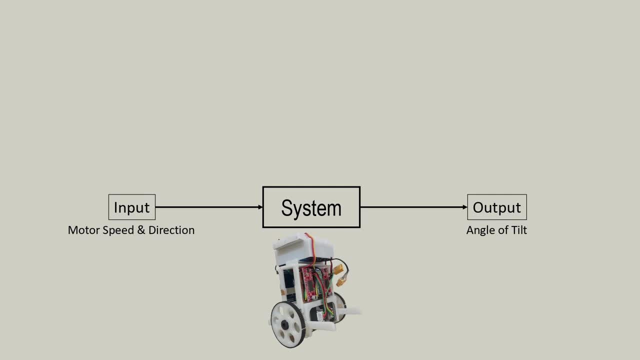 idea of a control system is to figure out how to generate the appropriate actuated signal, the input, so that our system will produce the desired controlled output. And that's basically the job of the control engineer: produce the right input into the system to get the output that you. 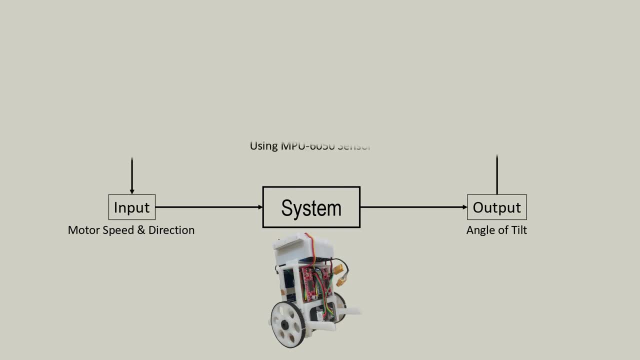 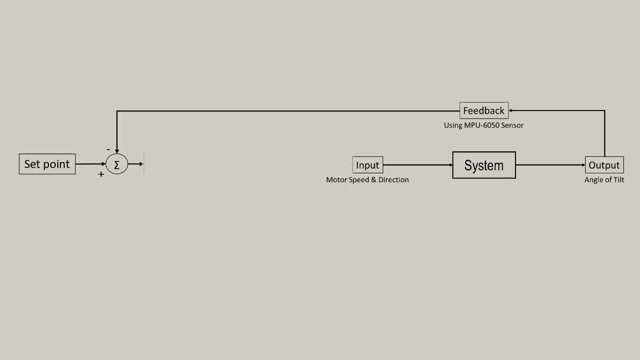 want, And in feedback control, the output of the system is fed back into the system- hence the name- and compared to the set point to see how far off the system is from where we want it to be. This difference between the two. 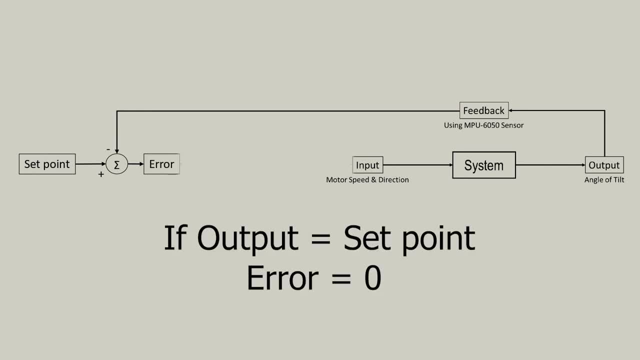 is the error term. If the output was exactly what we commanded it to be, then the error would go to zero, and that is what we want: zero error. So the question is: how do we take this error term and convert it into suitable actuator commands so that, over time, the error is driven to zero? 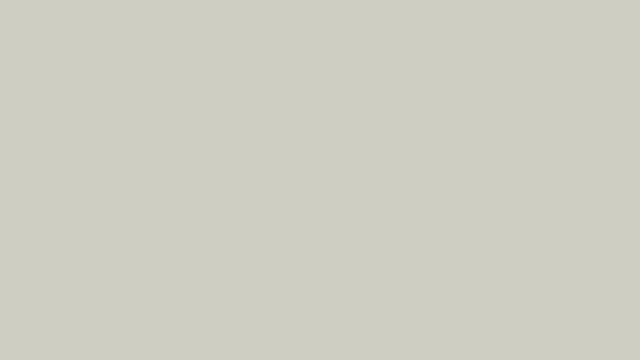 And the answer is with a controller. Now, let's say the desired angle of tilt is zero degrees, indicating an upright position. So let's say the desired angle of tilt is zero degrees, indicating an upright position At the beginning, if the robot is tilted, let's say 10 degrees to the 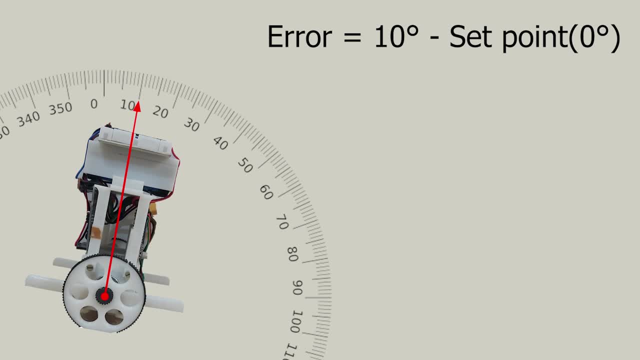 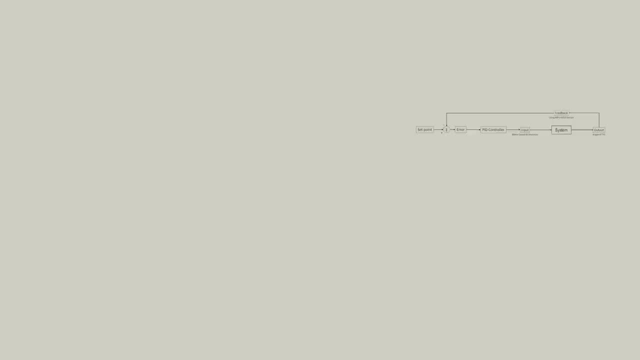 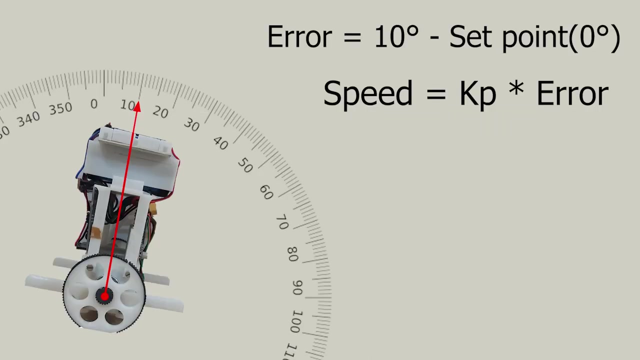 right, we have an error of 10 degrees. To balance the robot, we need to generate an appropriate actuated signal based on this error. Here we can use a PID controller. The proportional part of the controller will multiply the error by a gain value to determine the motor speed, For example.